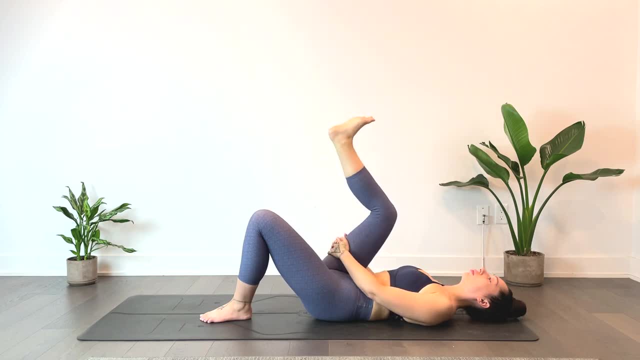 generous bend in that knee, Just as long as you continue to feel that stretch throughout the foot, the calf, and of course, feel free to skip any poses that do feel a bit too intense. No rules here, Honoring the body And we'll gently release. Placing that left ankle to the top of the right thigh and just 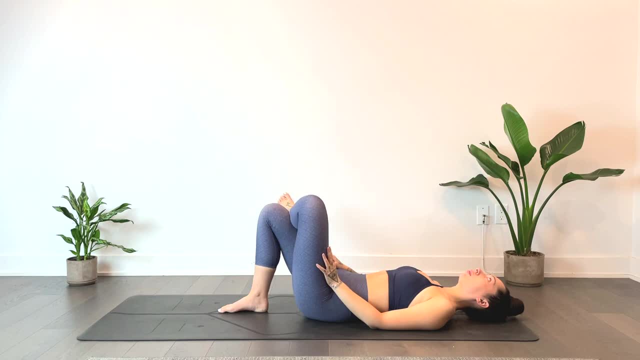 finding some movement within the foot. circling the foot And we'll gently release, Placing that left ankle to the top of the right thigh and just finding some movement within the foot. circling the foot And we'll gently release, Placing that left ankle to the top of the right thigh and just finding some movement within the foot. circling the foot. 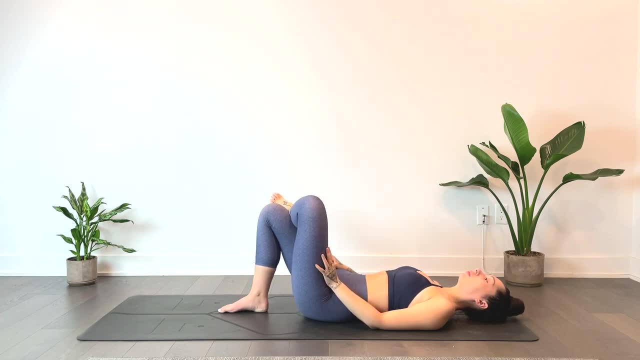 And we'll gently release Placing that left ankle to the top of the right thigh and just finding some movement within the foot circling the foot. And we'll gently release Placing that left ankle to the top of the right thigh and just finding some movement within the foot circling the foot. 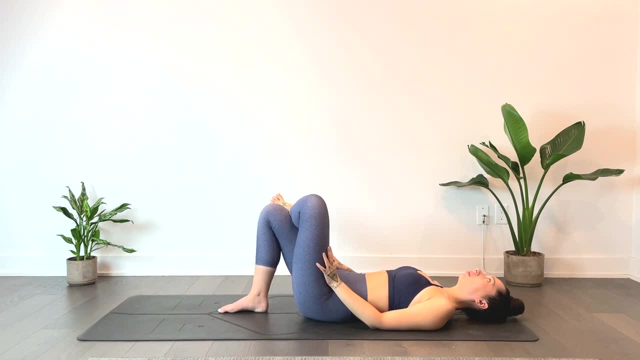 And we'll gently release Placing that left ankle to the top of the right thigh and just finding some movement within the foot circling the foot. And we'll gently release Placing that left ankle to the top of the right thigh and just finding some movement within the foot circling the foot. 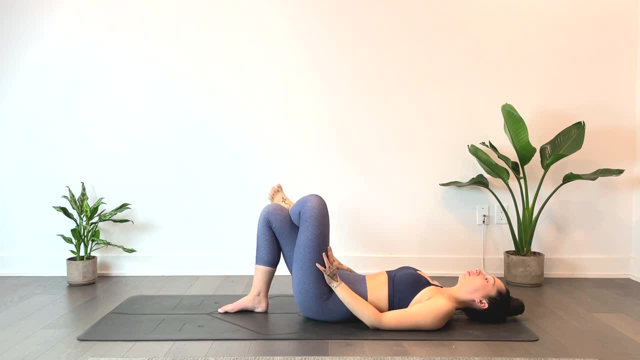 And we'll gently release Placing that left ankle to the top of the right thigh and just finding some movement within the foot circling the foot. And we'll gently release Placing that left ankle to the top of the right thigh and just finding some movement within the foot circling the foot. 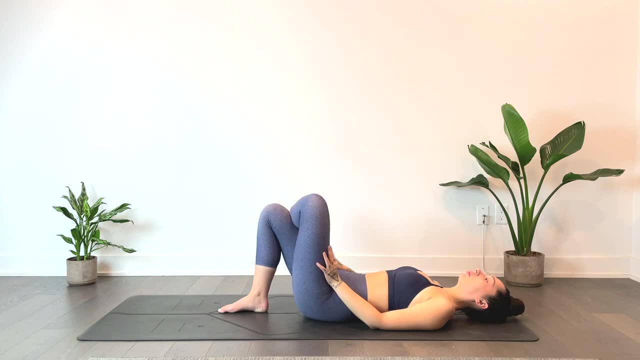 And we'll gently release Placing that left ankle to the top of the right thigh and just finding some movement within the foot circling the foot. And we'll gently release Placing that left ankle to the top of the right thigh and just finding some movement within the foot circling the foot. 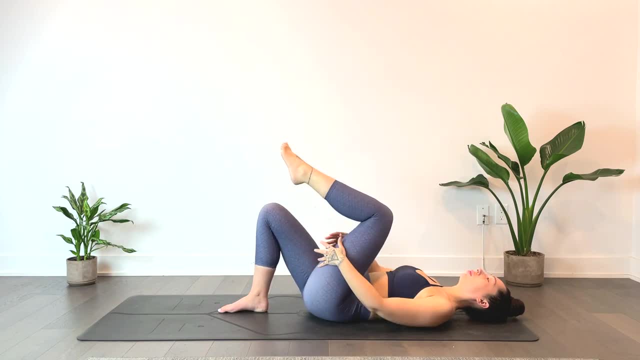 And we'll gently release Placing that left ankle to the top of the right thigh and just finding some movement within the foot circling the foot. And we'll gently release Placing that left ankle to the top of the right thigh and just finding some movement within the foot circling the foot. 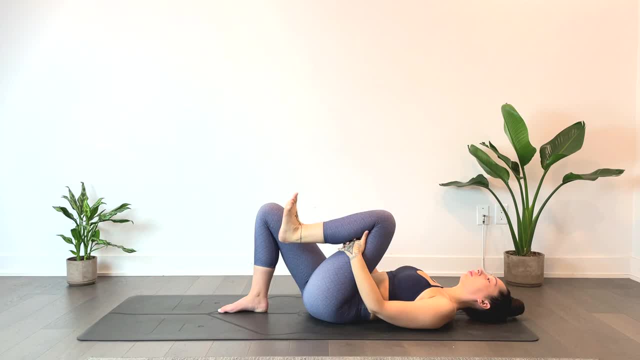 And we'll gently release Placing that left ankle to the top of the right thigh and just finding some movement within the foot circling the foot. And we'll gently release Placing that left ankle to the top of the right thigh and just finding some movement within the foot circling the foot. 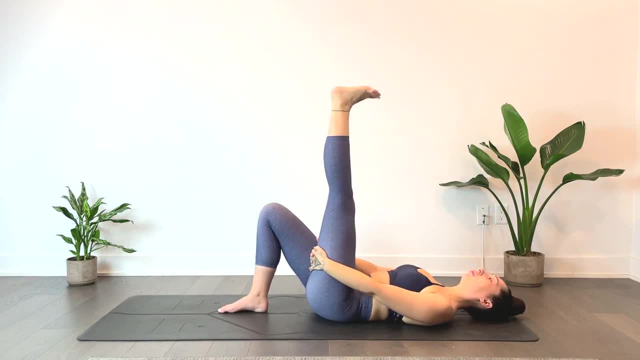 And we'll gently release Placing that left ankle to the top of the right thigh and just finding some movement within the foot circling the foot. And we'll gently release Placing that left ankle to the top of the right thigh and just finding some movement within the foot circling the foot. 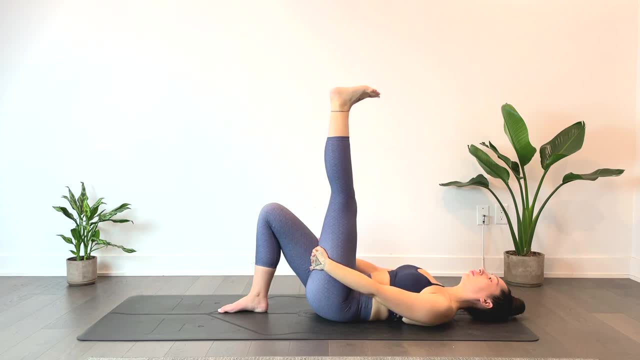 And we'll gently release Placing that left ankle to the top of the right thigh and just finding some movement within the foot circling the foot. And we'll gently release Placing that left ankle to the top of the right thigh and just finding some movement within the foot circling the foot. 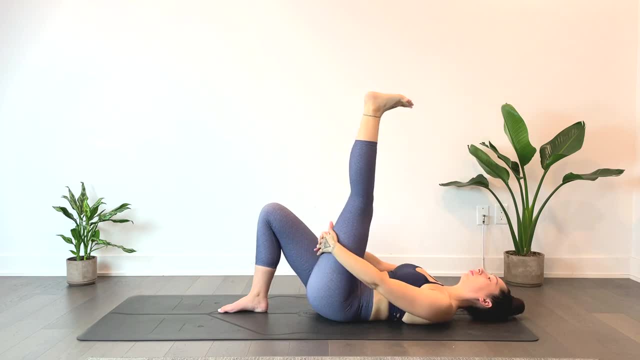 And we'll gently release Placing that left ankle to the top of the right thigh and just finding some movement within the foot circling the foot. And we'll gently release Placing that left ankle to the top of the right thigh and just finding some movement within the foot circling the foot. 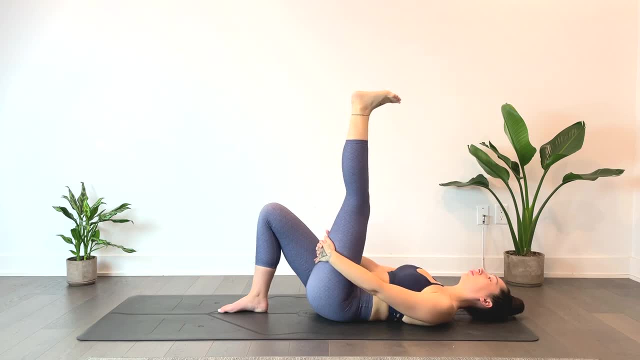 And we'll gently release Placing that left ankle to the top of the right thigh and just finding some movement within the foot circling the foot. And we'll gently release Placing that left ankle to the top of the right thigh and just finding some movement within the foot circling the foot. 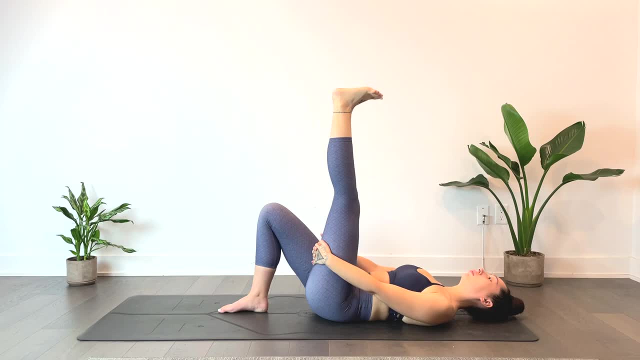 And we'll gently release Placing that left ankle to the top of the right thigh and just finding some movement within the foot circling the foot. And we'll gently release Placing that left ankle to the top of the right thigh and just finding some movement within the foot circling the foot. 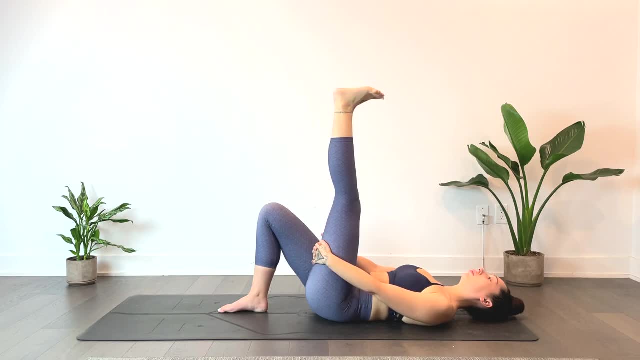 And we'll gently release Placing that left ankle to the top of the right thigh and just finding some movement within the foot circling the foot. And we'll gently release Placing that left ankle to the top of the right thigh and just finding some movement within the foot circling the foot. 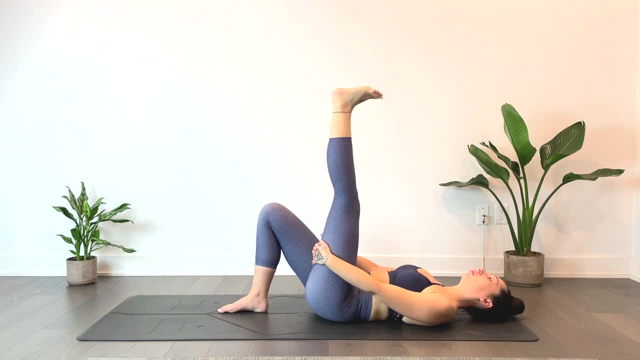 And we'll gently release Placing that left ankle to the top of the right thigh and just finding some movement within the foot circling the foot. And we'll gently release Placing that left ankle to the top of the right thigh and just finding some movement within the foot circling the foot. 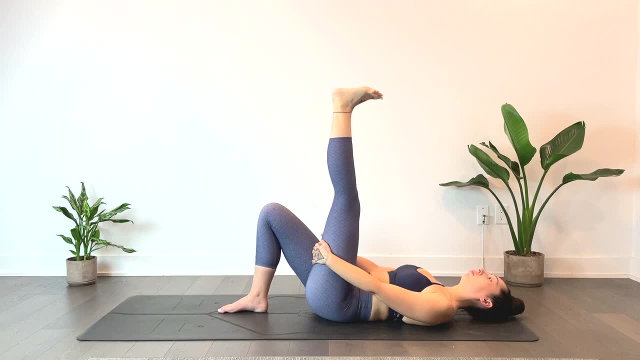 And we'll gently release Placing that left ankle to the top of the right thigh and just finding some movement within the foot circling the foot. And we'll gently release Placing that left ankle to the top of the right thigh and just finding some movement within the foot circling the foot. 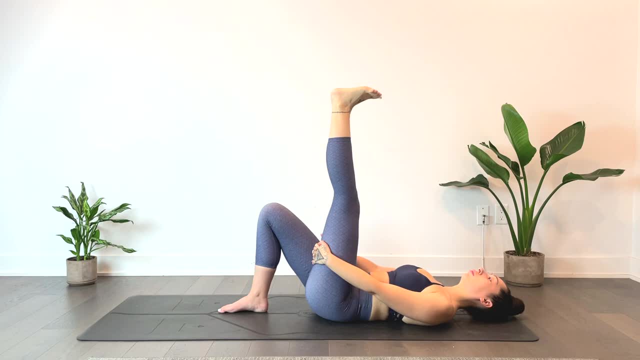 And we'll gently release Placing that left ankle to the top of the right thigh and just finding some movement within the foot circling the foot. And we'll gently release Placing that left ankle to the top of the right thigh and just finding some movement within the foot circling the foot. 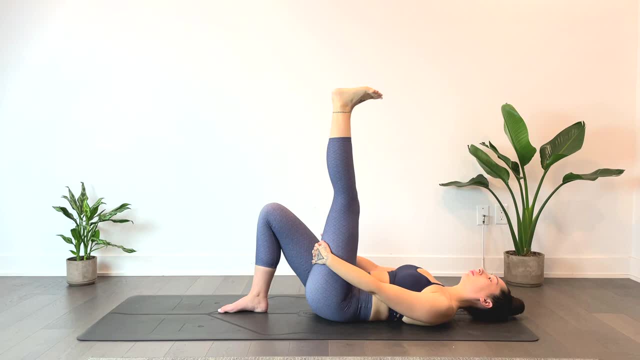 And we'll gently release Placing that left ankle to the top of the right thigh and just finding some movement within the foot circling the foot. And we'll gently release Placing that left ankle to the top of the right thigh and just finding some movement within the foot circling the foot. 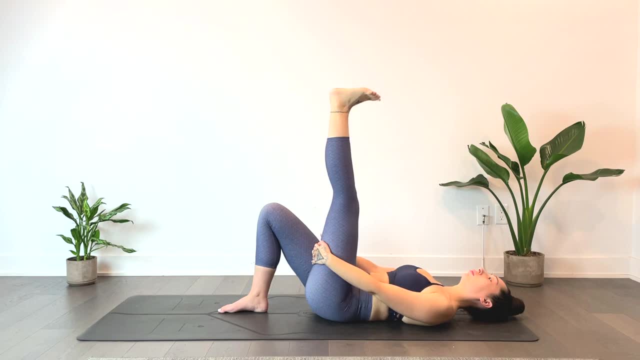 And we'll gently release Placing that left ankle to the top of the right thigh and just finding some movement within the foot circling the foot. And we'll gently release Placing that left ankle to the top of the right thigh and just finding some movement within the foot circling the foot. 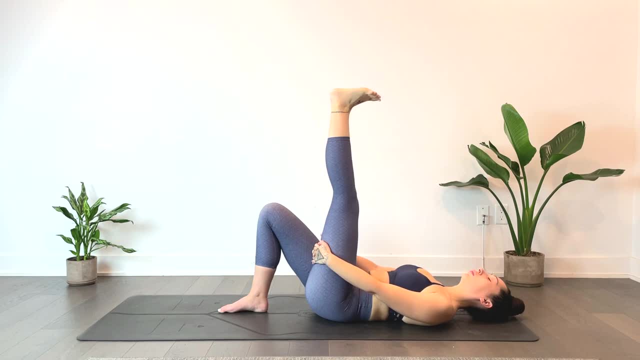 And we'll gently release Placing that left ankle to the top of the right thigh and just finding some movement within the foot circling the foot. And we'll gently release Placing that left ankle to the top of the right thigh and just finding some movement within the foot circling the foot. 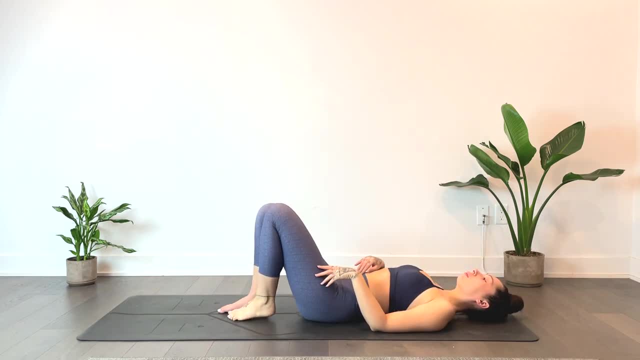 And we'll gently release Placing that left ankle to the top of the right thigh and just finding some movement within the foot circling the foot. And we'll gently release Placing that left ankle to the top of the right thigh and just finding some movement within the foot circling the foot. 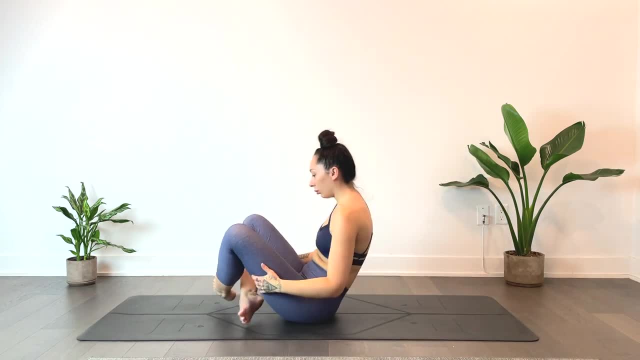 And we'll gently release Placing that left ankle to the top of the right thigh and just finding some movement within the foot circling the foot. And we'll gently release Placing that left ankle to the top of the right thigh and just finding some movement within the foot circling the foot. 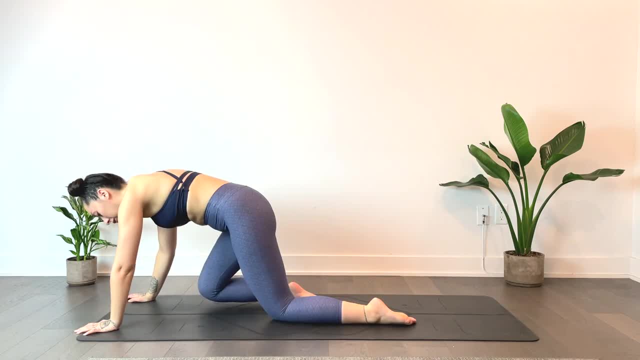 And we'll gently release Placing that left ankle to the top of the right thigh and just finding some movement within the foot circling the foot. And we'll gently release Placing that left ankle to the top of the right thigh and just finding some movement within the foot circling the foot. 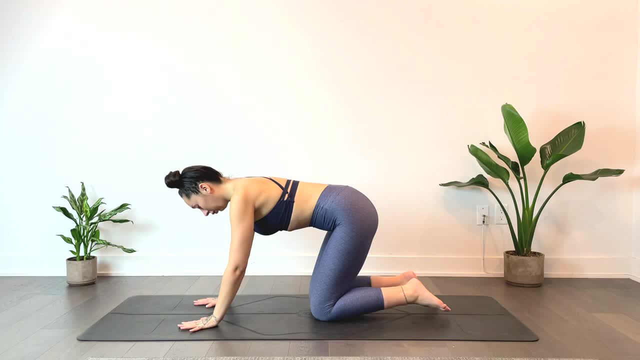 And we'll gently release Placing that left ankle to the top of the right thigh and just finding some movement within the foot circling the foot. And we'll gently release Placing that left ankle to the top of the right thigh and just finding some movement within the foot circling the foot. 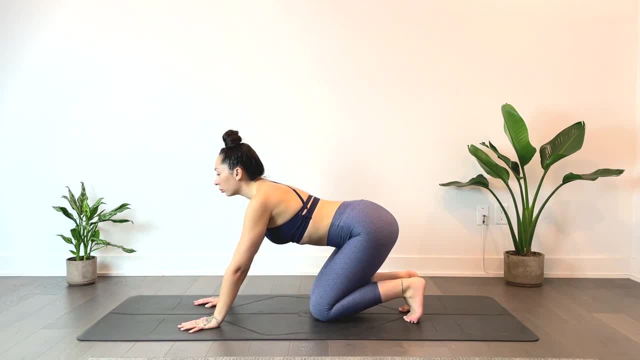 And we'll gently release Placing that left ankle to the top of the right thigh and just finding some movement within the foot circling the foot. And we'll gently release Placing that left ankle to the top of the right thigh and just finding some movement within the foot circling the foot. 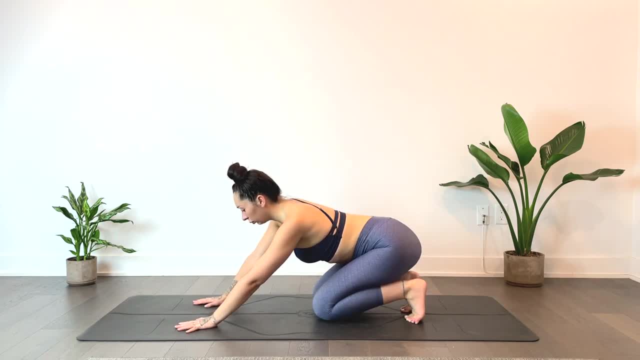 And we'll gently release Placing that left ankle to the top of the right thigh and just finding some movement within the foot circling the foot. And we'll gently release Placing that left ankle to the top of the right thigh and just finding some movement within the foot circling the foot. 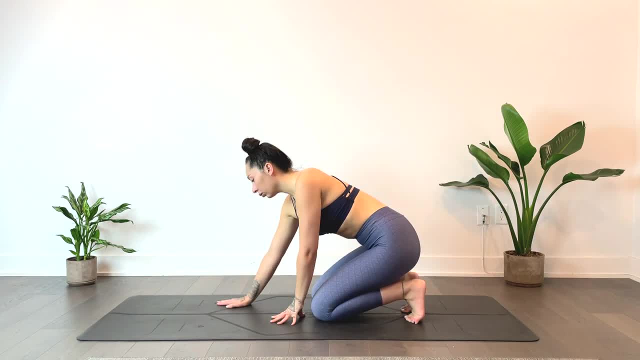 And we'll gently release Placing that left ankle to the top of the right thigh and just finding some movement within the foot circling the foot. And we'll gently release Placing that left ankle to the top of the right thigh and just finding some movement within the foot circling the foot. 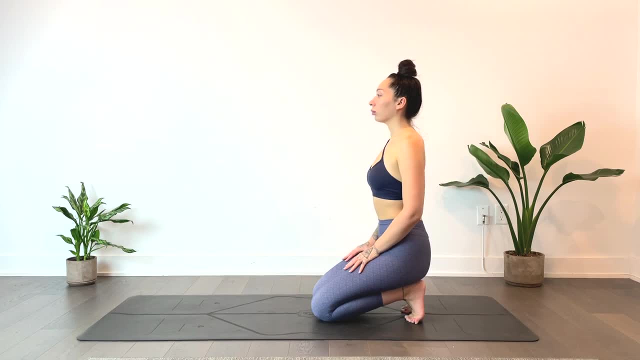 And we'll gently release Placing that left ankle to the top of the right thigh and just finding some movement within the foot circling the foot. And we'll gently release Placing that left ankle to the top of the right thigh and just finding some movement within the foot circling the foot. 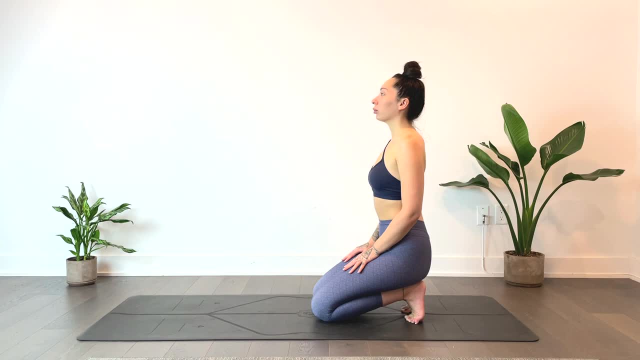 And we'll gently release Placing that left ankle to the top of the right thigh and just finding some movement within the foot circling the foot. And we'll gently release Placing that left ankle to the top of the right thigh and just finding some movement within the foot circling the foot. 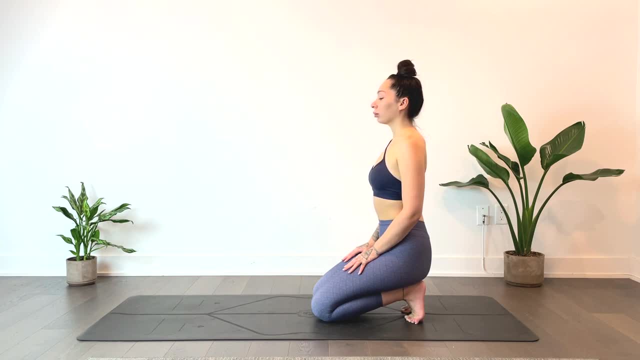 And we'll gently release Placing that left ankle to the top of the right thigh and just finding some movement within the foot circling the foot. And we'll gently release Placing that left ankle to the top of the right thigh and just finding some movement within the foot circling the foot. 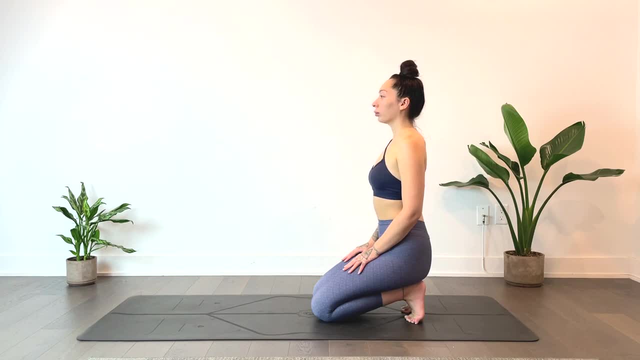 And we'll gently release Placing that left ankle to the top of the right thigh and just finding some movement within the foot circling the foot. And we'll gently release Placing that left ankle to the top of the right thigh and just finding some movement within the foot circling the foot. 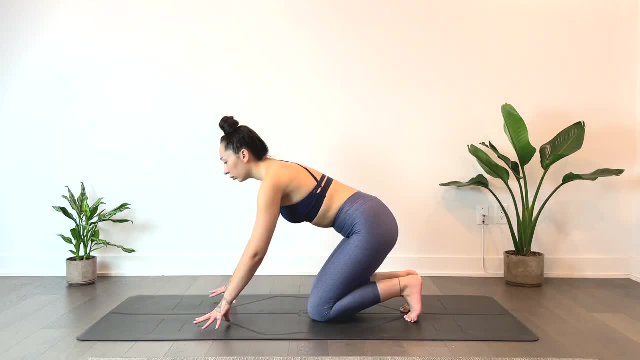 And we'll gently release Placing that left ankle to the top of the right thigh and just finding some movement within the foot circling the foot. And we'll gently release Placing that left ankle to the top of the right thigh and just finding some movement within the foot circling the foot. 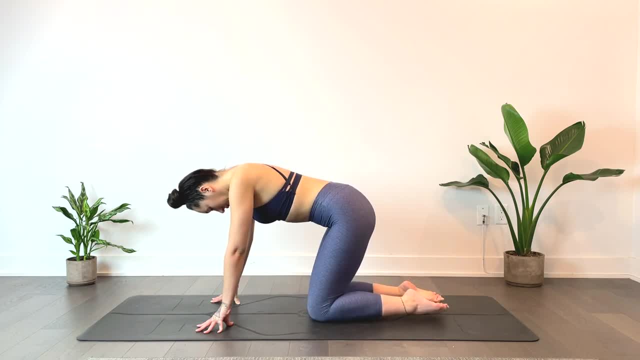 And we'll gently release Placing that left ankle to the top of the right thigh and just finding some movement within the foot circling the foot. And we'll gently release Placing that left ankle to the top of the right thigh and just finding some movement within the foot circling the foot. 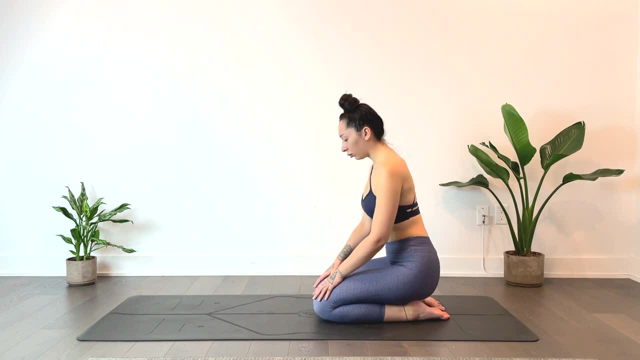 And we'll gently release Placing that left ankle to the top of the right thigh and just finding some movement within the foot circling the foot. And we'll gently release Placing that left ankle to the top of the right thigh and just finding some movement within the foot circling the foot. 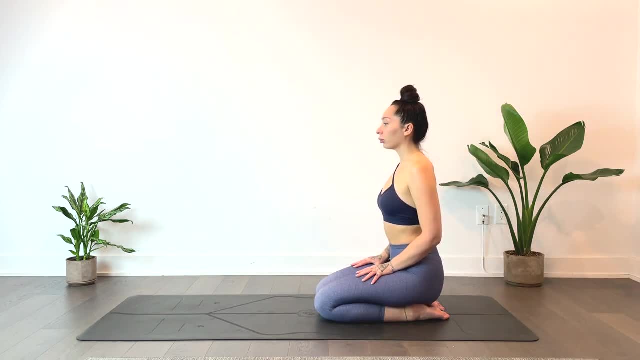 And we'll gently release Placing that left ankle to the top of the right thigh and just finding some movement within the foot circling the foot. And we'll gently release Placing that left ankle to the top of the right thigh and just finding some movement within the foot circling the foot. 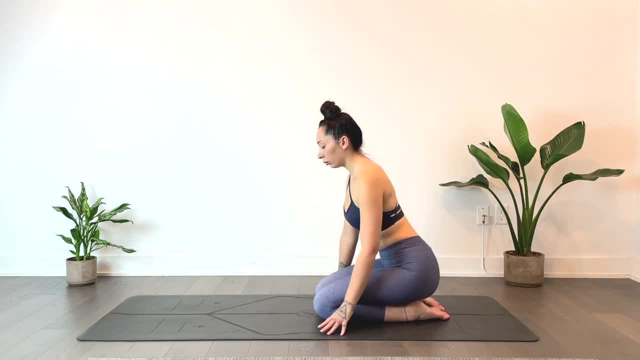 And we'll gently release Placing that left ankle to the top of the right thigh and just finding some movement within the foot circling the foot. And we'll gently release Placing that left ankle to the top of the right thigh and just finding some movement within the foot circling the foot. 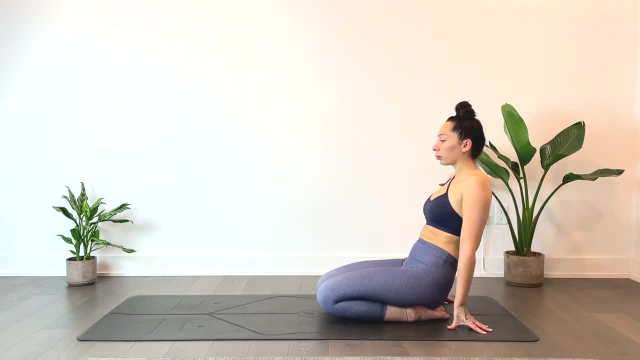 And we'll gently release Placing that left ankle to the top of the right thigh and just finding some movement within the foot circling the foot. And we'll gently release Placing that left ankle to the top of the right thigh and just finding some movement within the foot circling the foot. 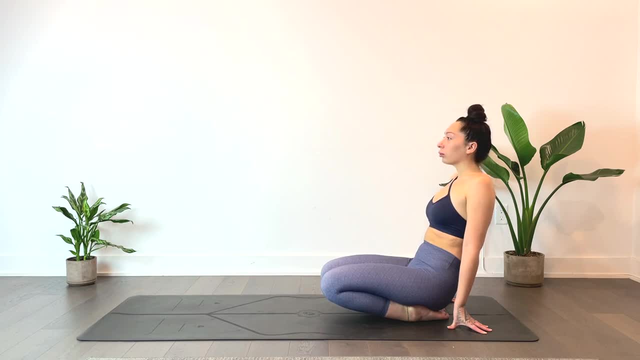 And we'll gently release Placing that left ankle to the top of the right thigh and just finding some movement within the foot circling the foot. And we'll gently release Placing that left ankle to the top of the right thigh and just finding some movement within the foot circling the foot. 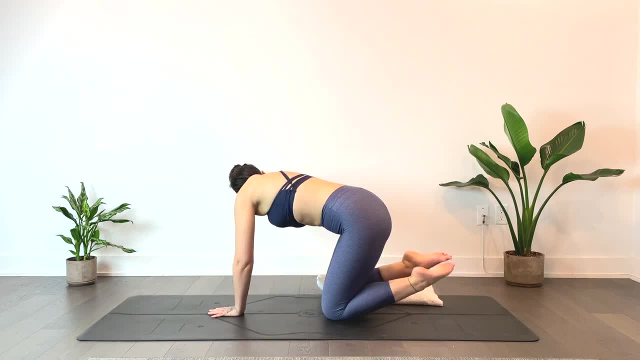 And we'll gently release Placing that left ankle to the top of the right thigh and just finding some movement within the foot circling the foot. And we'll gently release Placing that left ankle to the top of the right thigh and just finding some movement within the foot circling the foot. 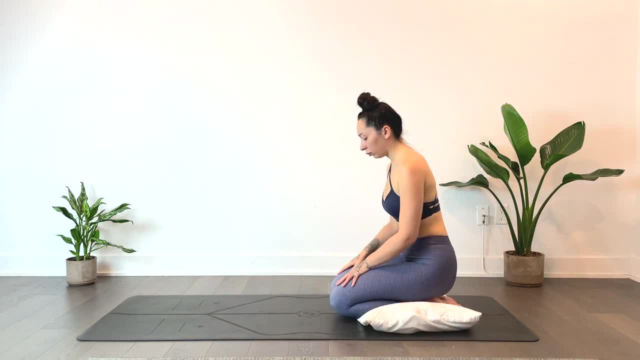 And we'll gently release Placing that left ankle to the top of the right thigh and just finding some movement within the foot circling the foot. And we'll gently release Placing that left ankle to the top of the right thigh and just finding some movement within the foot circling the foot. 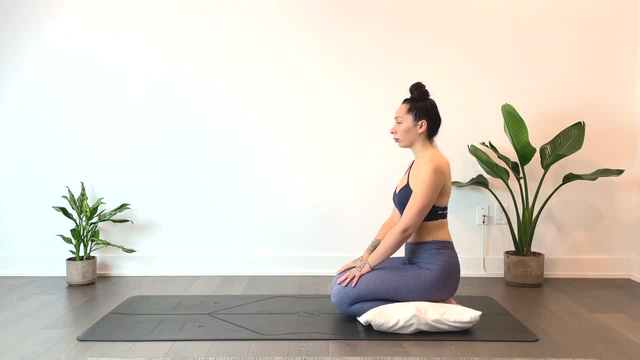 And we'll gently release Placing that left ankle to the top of the right thigh and just finding some movement within the foot circling the foot. And we'll gently release Placing that left ankle to the top of the right thigh and just finding some movement within the foot circling the foot. 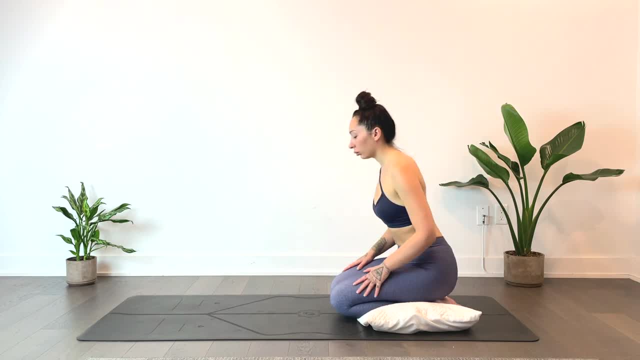 And we'll gently release Placing that left ankle to the top of the right thigh and just finding some movement within the foot circling the foot. And we'll gently release Placing that left ankle to the top of the right thigh and just finding some movement within the foot circling the foot. 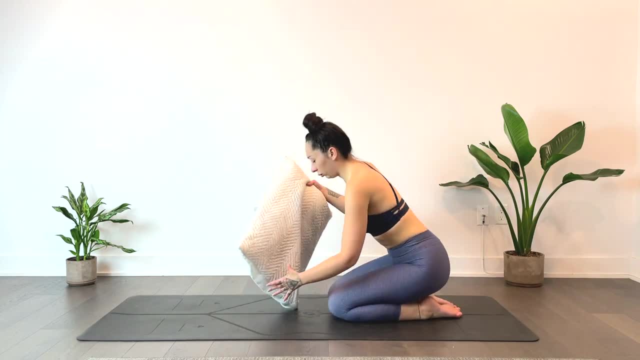 And we'll gently release Placing that left ankle to the top of the right thigh and just finding some movement within the foot circling the foot. And we'll gently release Placing that left ankle to the top of the right thigh and just finding some movement within the foot circling the foot. 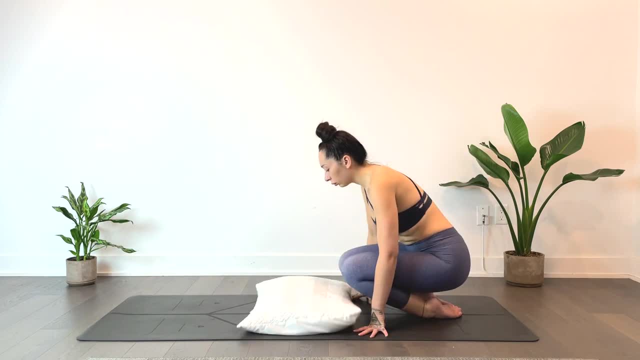 And we'll gently release Placing that left ankle to the top of the right thigh and just finding some movement within the foot circling the foot. And we'll gently release Placing that left ankle to the top of the right thigh and just finding some movement within the foot circling the foot. 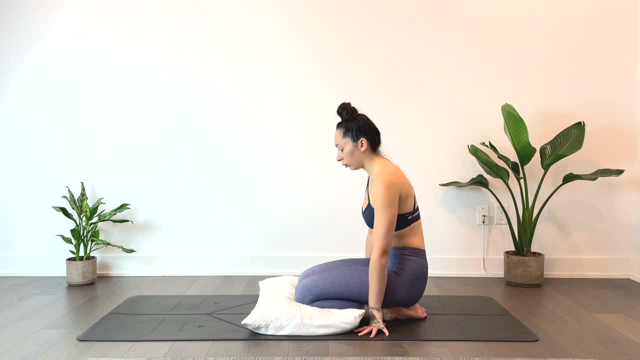 And we'll gently release Placing that left ankle to the top of the right thigh and just finding some movement within the foot circling the foot. And we'll gently release Placing that left ankle to the top of the right thigh and just finding some movement within the foot circling the foot. 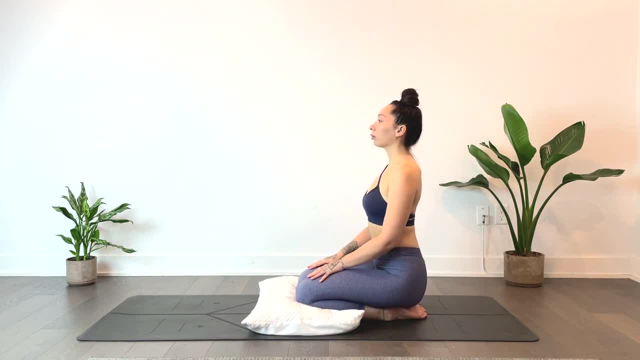 And we'll gently release Placing that left ankle to the top of the right thigh and just finding some movement within the foot circling the foot. And we'll gently release Placing that left ankle to the top of the right thigh and just finding some movement within the foot circling the foot. 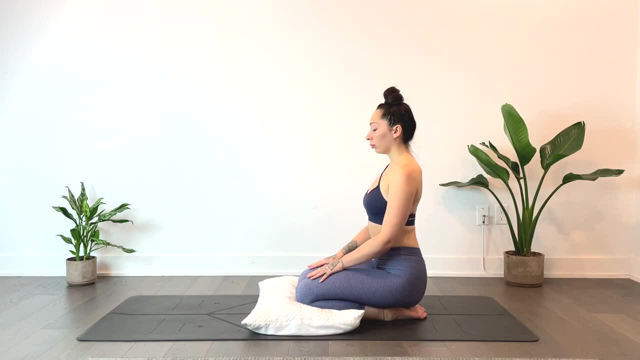 And we'll gently release Placing that left ankle to the top of the right thigh and just finding some movement within the foot circling the foot. And we'll gently release Placing that left ankle to the top of the right thigh and just finding some movement within the foot circling the foot. 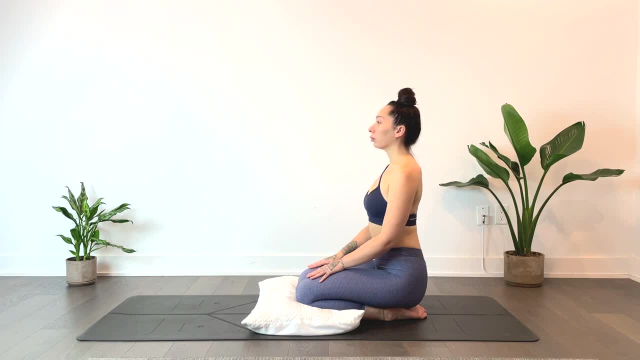 And we'll gently release Placing that left ankle to the top of the right thigh and just finding some movement within the foot circling the foot. And we'll gently release Placing that left ankle to the top of the right thigh and just finding some movement within the foot circling the foot. 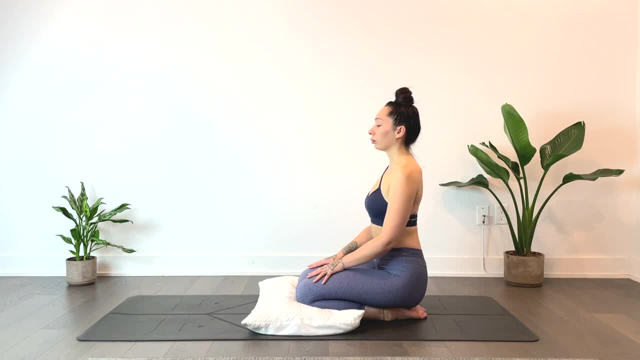 And we'll gently release Placing that left ankle to the top of the right thigh and just finding some movement within the foot circling the foot. And we'll gently release Placing that left ankle to the top of the right thigh and just finding some movement within the foot circling the foot. 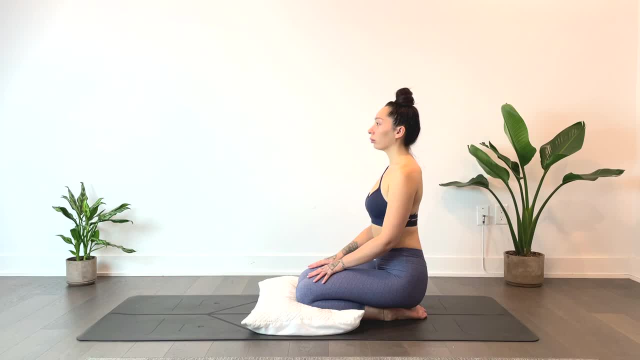 And we'll gently release Placing that left ankle to the top of the right thigh and just finding some movement within the foot circling the foot. And we'll gently release Placing that left ankle to the top of the right thigh and just finding some movement within the foot circling the foot. 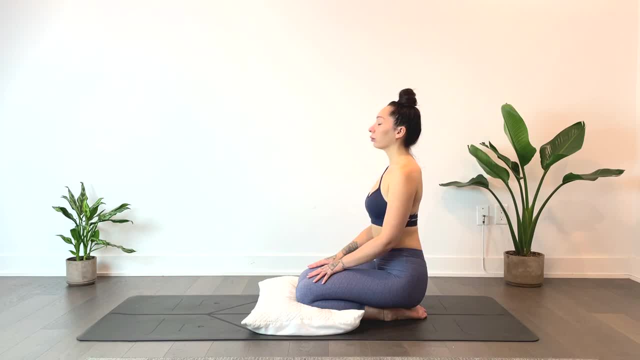 And we'll gently release Placing that left ankle to the top of the right thigh and just finding some movement within the foot circling the foot. And we'll gently release Placing that left ankle to the top of the right thigh and just finding some movement within the foot circling the foot. 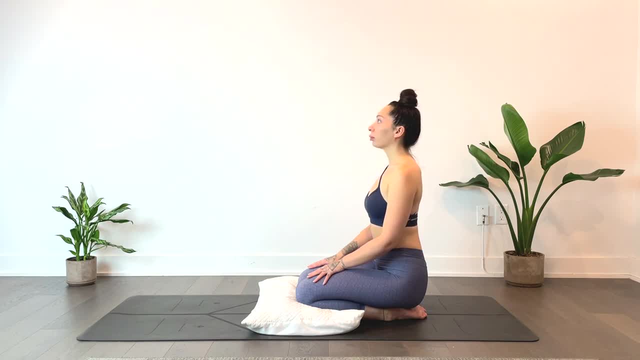 And we'll gently release Placing that left ankle to the top of the right thigh and just finding some movement within the foot circling the foot. And we'll gently release Placing that left ankle to the top of the right thigh and just finding some movement within the foot circling the foot. 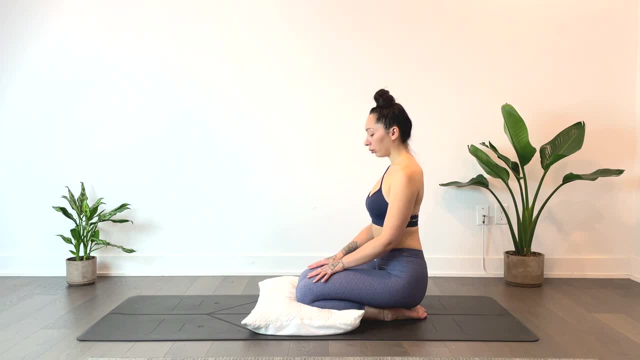 And we'll gently release Placing that left ankle to the top of the right thigh and just finding some movement within the foot circling the foot. And we'll gently release Placing that left ankle to the top of the right thigh and just finding some movement within the foot circling the foot. 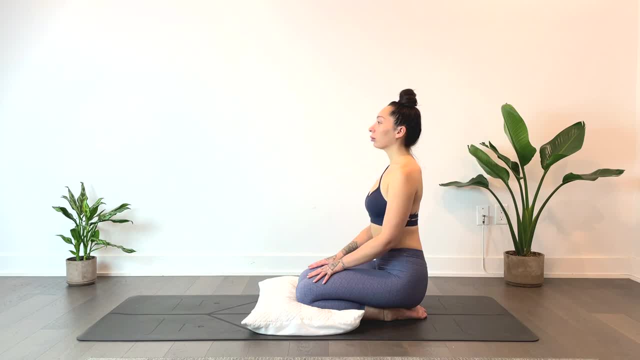 And we'll gently release Placing that left ankle to the top of the right thigh and just finding some movement within the foot circling the foot. And we'll gently release Placing that left ankle to the top of the right thigh and just finding some movement within the foot circling the foot. 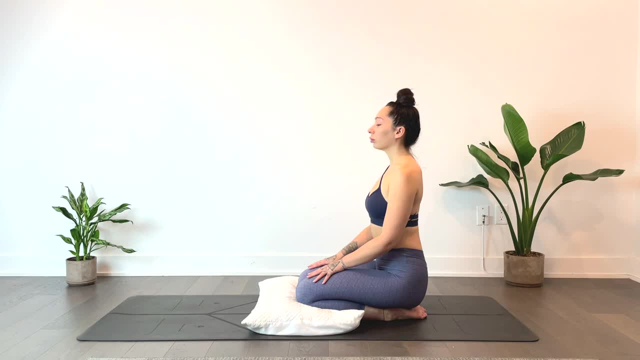 And we'll gently release Placing that left ankle to the top of the right thigh and just finding some movement within the foot circling the foot. And we'll gently release Placing that left ankle to the top of the right thigh and just finding some movement within the foot circling the foot. 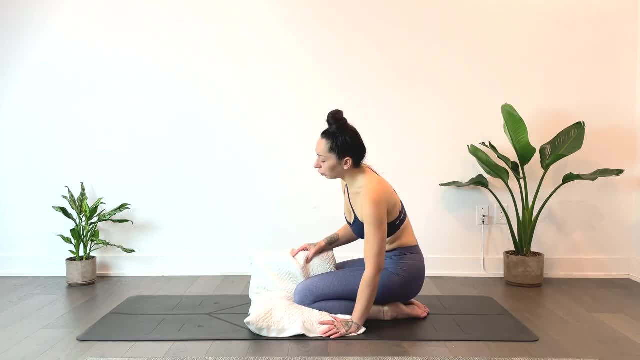 And we'll gently release Placing that left ankle to the top of the right thigh and just finding some movement within the foot circling the foot. And we'll gently release Placing that left ankle to the top of the right thigh and just finding some movement within the foot circling the foot. 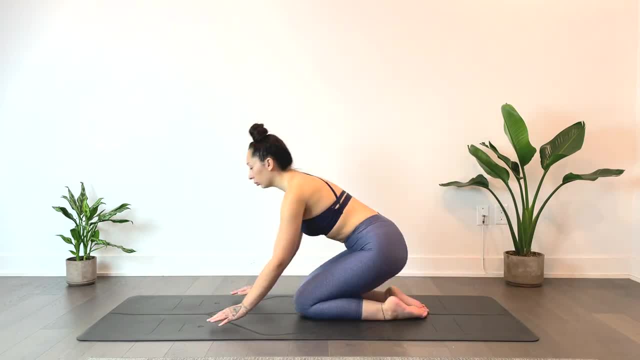 And we'll gently release Placing that left ankle to the top of the right thigh and just finding some movement within the foot circling the foot. And we'll gently release Placing that left ankle to the top of the right thigh and just finding some movement within the foot circling the foot. 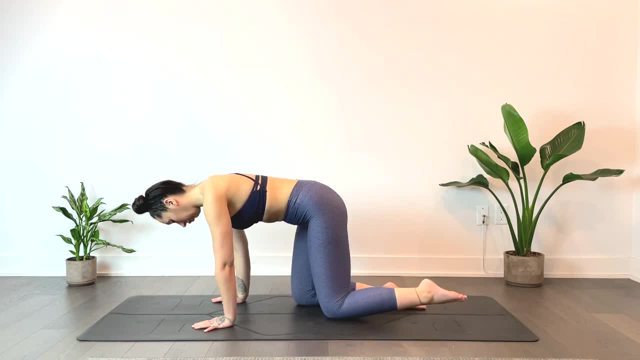 And we'll gently release Placing that left ankle to the top of the right thigh and just finding some movement within the foot circling the foot. And we'll gently release Placing that left ankle to the top of the right thigh and just finding some movement within the foot circling the foot. 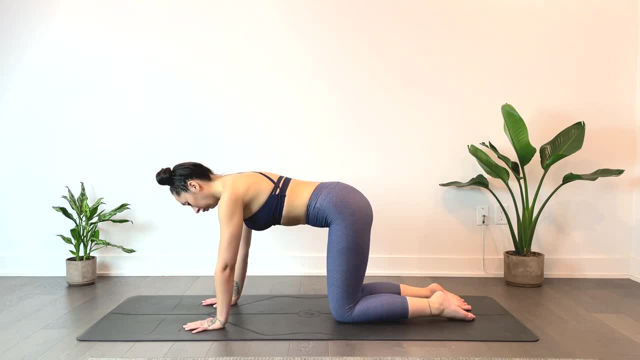 And we'll gently release Placing that left ankle to the top of the right thigh and just finding some movement within the foot circling the foot. And we'll gently release Placing that left ankle to the top of the right thigh and just finding some movement within the foot circling the foot. 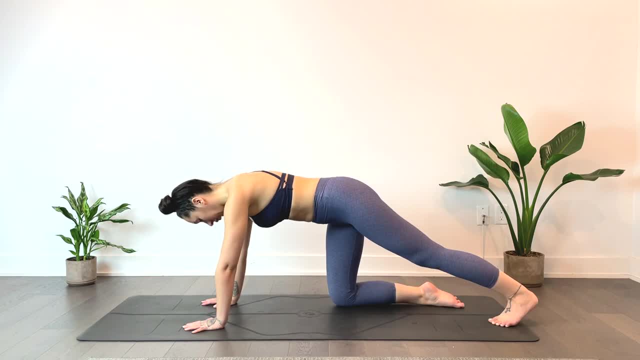 And we'll gently release Placing that left ankle to the top of the right thigh and just finding some movement within the foot circling the foot. And we'll gently release Placing that left ankle to the top of the right thigh and just finding some movement within the foot circling the foot. 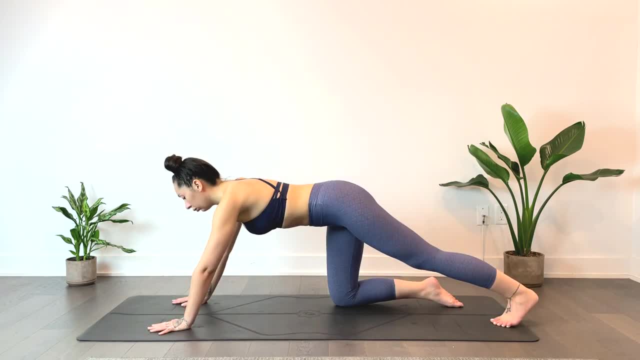 And we'll gently release Placing that left ankle to the top of the right thigh and just finding some movement within the foot circling the foot. And we'll gently release Placing that left ankle to the top of the right thigh and just finding some movement within the foot circling the foot. 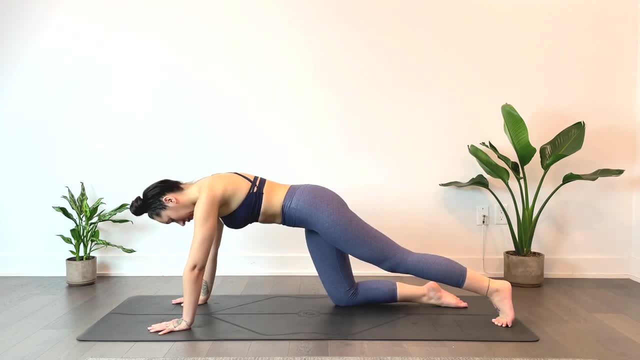 And we'll gently release Placing that left ankle to the top of the right thigh and just finding some movement within the foot circling the foot. And we'll gently release Placing that left ankle to the top of the right thigh and just finding some movement within the foot circling the foot. 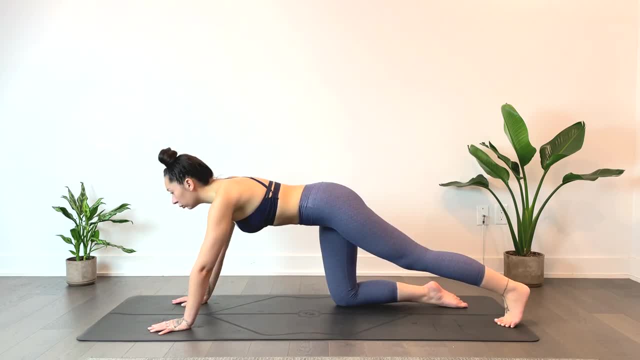 And we'll gently release Placing that left ankle to the top of the right thigh and just finding some movement within the foot circling the foot. And we'll gently release Placing that left ankle to the top of the right thigh and just finding some movement within the foot circling the foot. 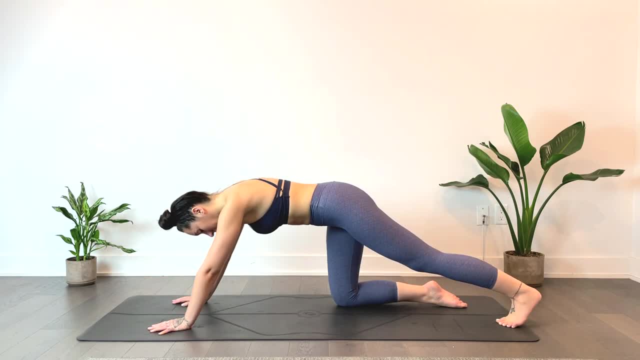 And we'll gently release Placing that left ankle to the top of the right thigh and just finding some movement within the foot circling the foot. And we'll gently release Placing that left ankle to the top of the right thigh and just finding some movement within the foot circling the foot. 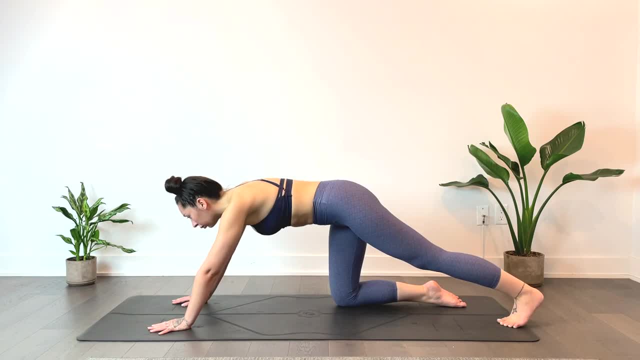 And we'll gently release Placing that left ankle to the top of the right thigh and just finding some movement within the foot circling the foot. And we'll gently release Placing that left ankle to the top of the right thigh and just finding some movement within the foot circling the foot. 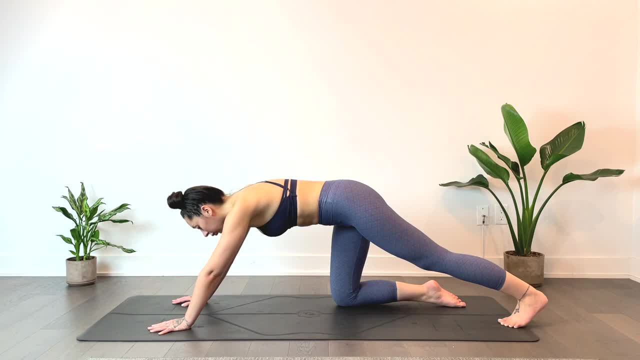 And we'll gently release Placing that left ankle to the top of the right thigh and just finding some movement within the foot circling the foot. And we'll gently release Placing that left ankle to the top of the right thigh and just finding some movement within the foot circling the foot. 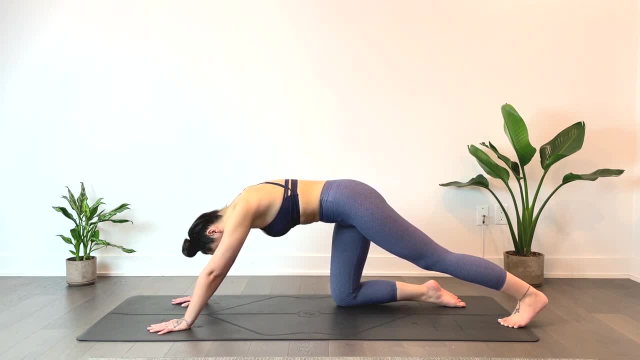 And we'll gently release Placing that left ankle to the top of the right thigh and just finding some movement within the foot circling the foot. And we'll gently release Placing that left ankle to the top of the right thigh and just finding some movement within the foot circling the foot. 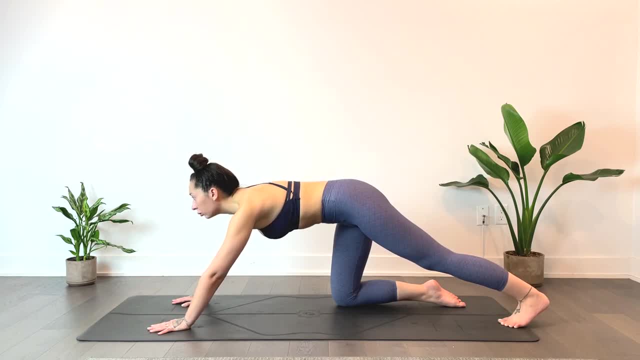 And we'll gently release Placing that left ankle to the top of the right thigh and just finding some movement within the foot circling the foot. And we'll gently release Placing that left ankle to the top of the right thigh and just finding some movement within the foot circling the foot. 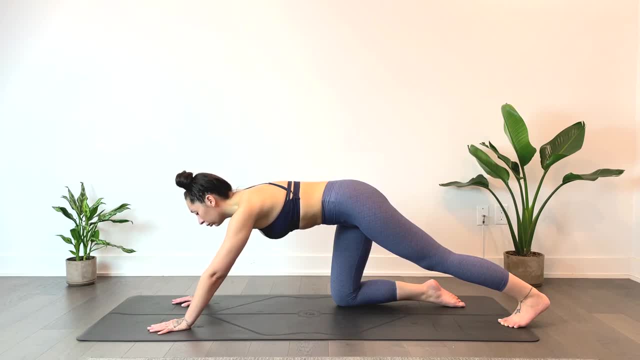 And we'll gently release Placing that left ankle to the top of the right thigh and just finding some movement within the foot circling the foot. And we'll gently release Placing that left ankle to the top of the right thigh and just finding some movement within the foot circling the foot. 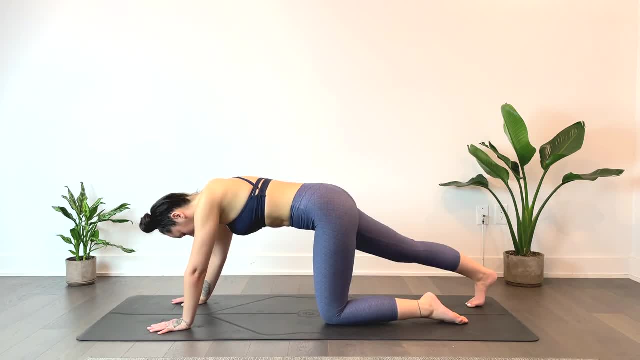 And we'll gently release Placing that left ankle to the top of the right thigh and just finding some movement within the foot circling the foot. And we'll gently release Placing that left ankle to the top of the right thigh and just finding some movement within the foot circling the foot. 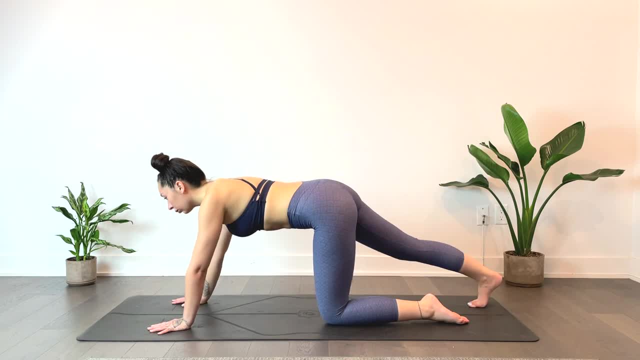 And we'll gently release Placing that left ankle to the top of the right thigh and just finding some movement within the foot circling the foot. And we'll gently release Placing that left ankle to the top of the right thigh and just finding some movement within the foot circling the foot. 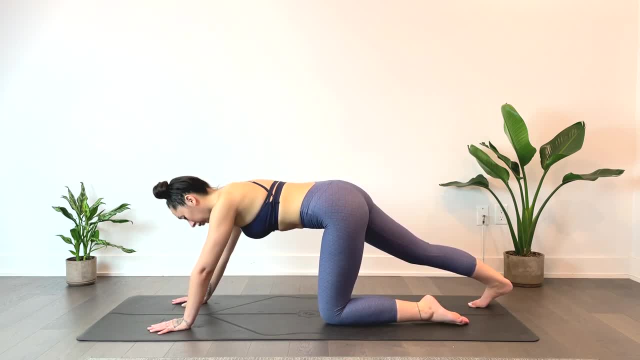 And we'll gently release Placing that left ankle to the top of the right thigh and just finding some movement within the foot circling the foot. And we'll gently release Placing that left ankle to the top of the right thigh and just finding some movement within the foot circling the foot. 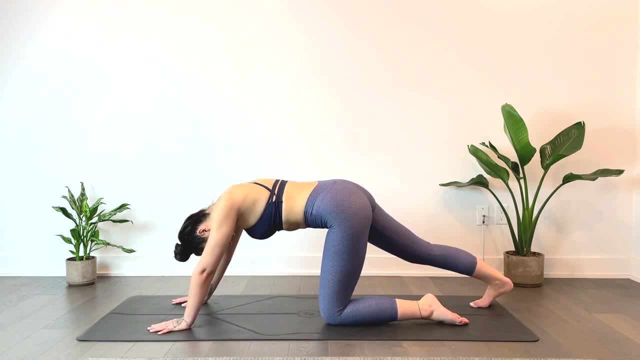 And we'll gently release Placing that left ankle to the top of the right thigh and just finding some movement within the foot circling the foot. And we'll gently release Placing that left ankle to the top of the right thigh and just finding some movement within the foot circling the foot. 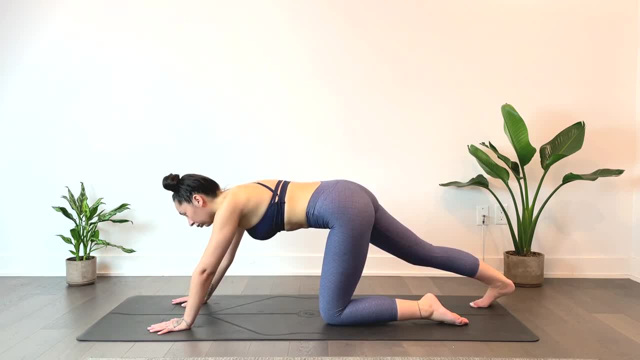 And we'll gently release Placing that left ankle to the top of the right thigh and just finding some movement within the foot circling the foot. And we'll gently release Placing that left ankle to the top of the right thigh and just finding some movement within the foot circling the foot. 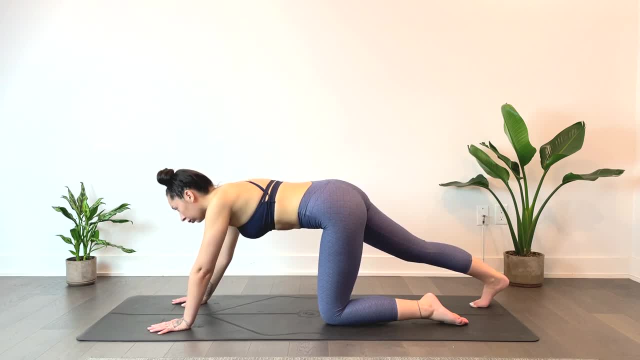 And we'll gently release Placing that left ankle to the top of the right thigh and just finding some movement within the foot circling the foot. And we'll gently release Placing that left ankle to the top of the right thigh and just finding some movement within the foot circling the foot. 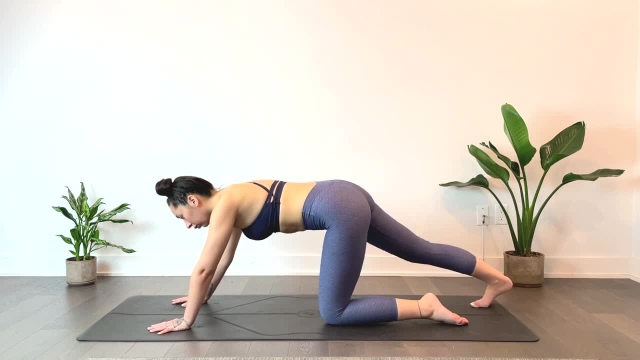 And we'll gently release Placing that left ankle to the top of the right thigh and just finding some movement within the foot. circling the foot. We'll gently release sending the hips towards the heels, forehead or cheek to the mat for